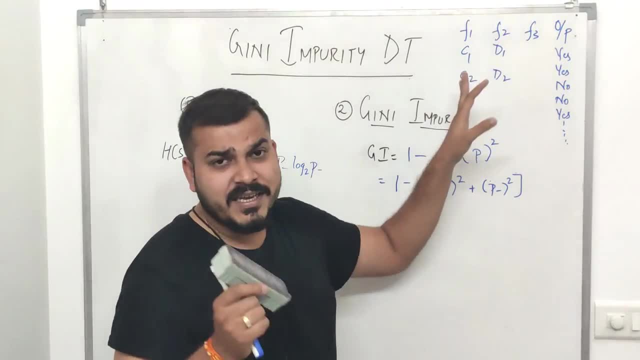 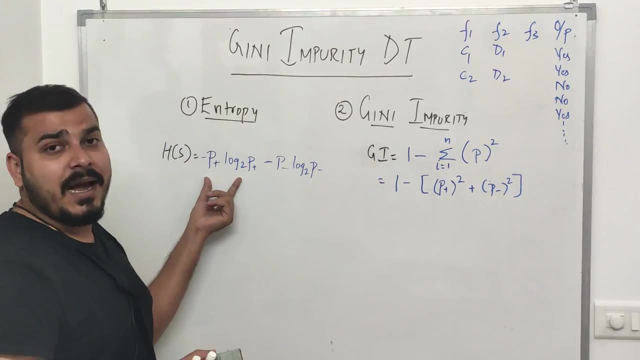 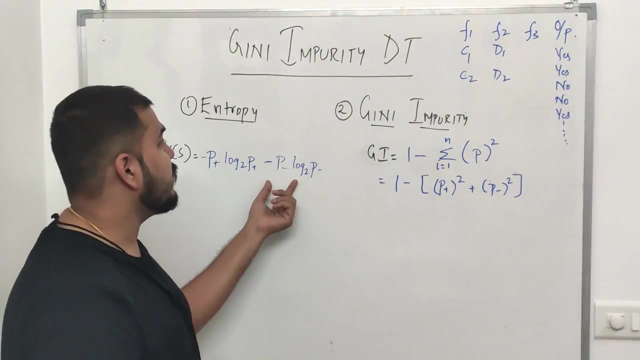 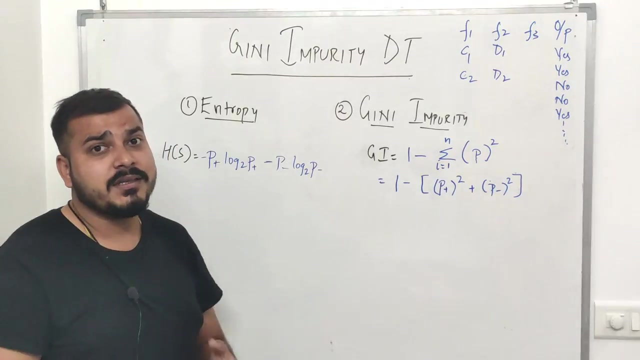 like C1, C2, D1, D2, D3, something like that. I'm just taking it as an example And the output is a binary classifier like yes or no. Okay, Now, in this particular case, I'm saying that P plus is basically the number of time, the percentage of values that has basically yes, Okay, P minus is basically the number of values that has actually no, Okay, So we are going to consider this particular equation. I've already explained you about this in my previous video. Right, So this is all about entropy. Now, in entropy, what we used to do is that, suppose. 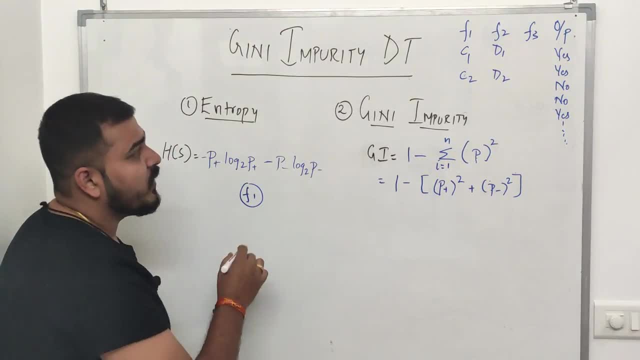 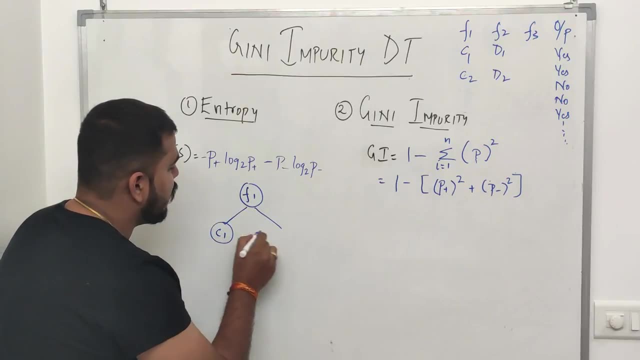 I select F1, right F1- as my root node, Then what it does is that it will go and find out how many category variables are there inside it. So, based on that, we'll be creating two nodes. So right now, 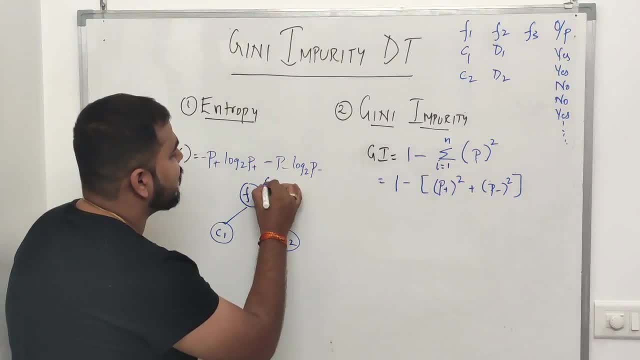 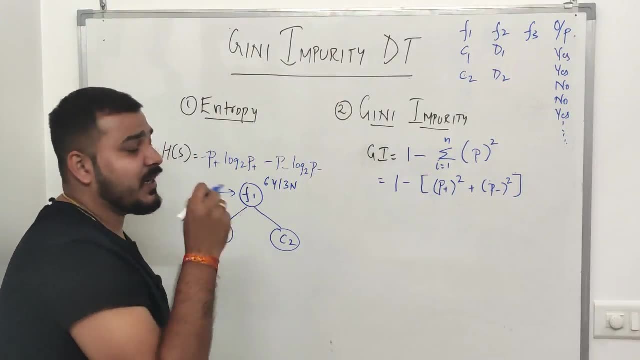 we have C1 and C2.. Suppose consider that I had over here 6 yes and 3 no's. The total number of output of yes and no when I was seeing at this particular point, at this particular root node, it was 6 yes and 3 no. Now, after the split, suppose I got over here as 3 yes, 3 no's. 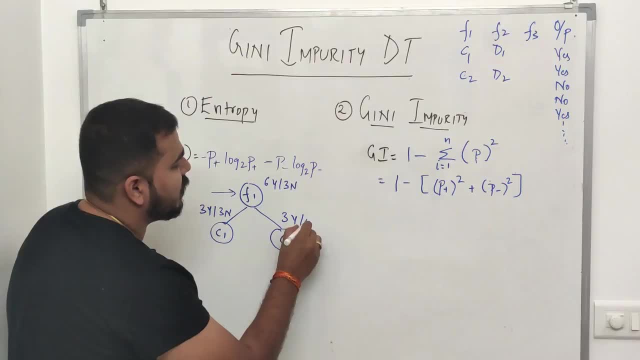 Right, And after this particular split, again I got 3 yes and 0 no's. Now, when I see the 0 no's, this basically becomes a leaf node. Okay, This basically becomes a leaf node. Pretty much simple. 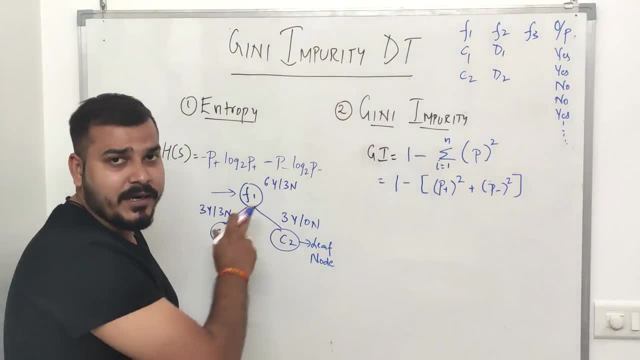 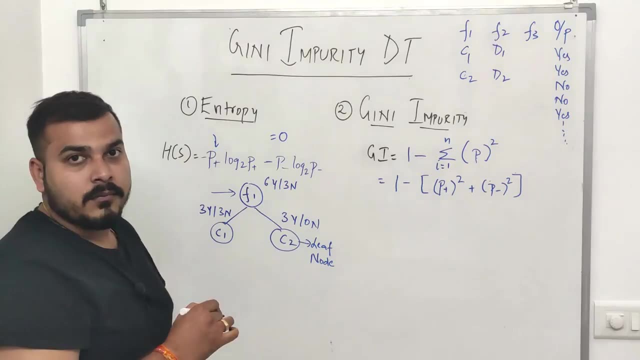 Right Now why it is leaf node? Because here I'm getting a pure split Right Now. if I try to compute this with respect to this particular entropy, my value will be 0. How Just understand guys. minus P, minus, minus P, plus P, plus over here basically means probably. 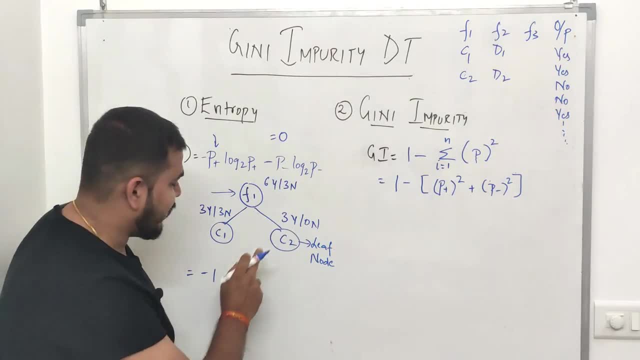 percentage of yes values. Total number of yes values is 3.. So 3 divided by 0.. Right Percentage. I'll actually calculate the sum. Sorry, it should not be 0. It should be 3. 3 divided by 3. Right. 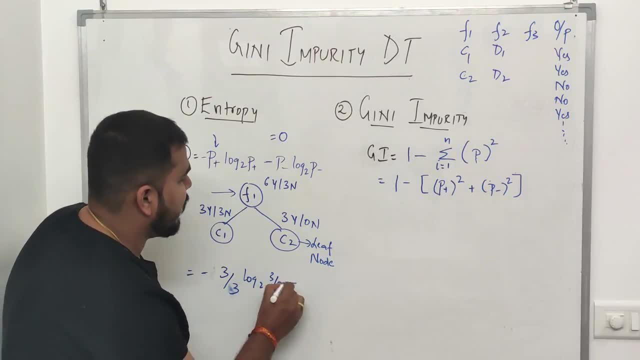 Log of base 2, 3 divided by 3, minus. What is P minus? Now we need to understand what is P minus. Over here I see 0, no's Right. So my 0 value divided by 3, log base 2, 0 by 3.. So this is how. 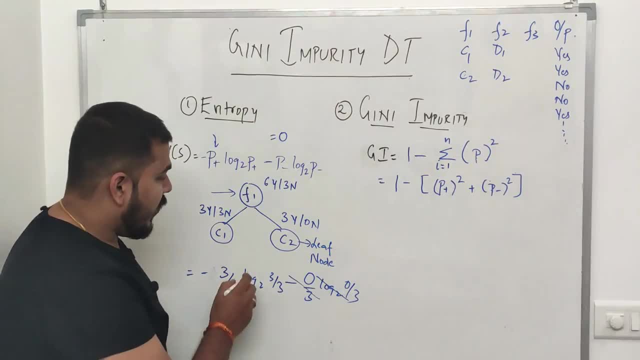 the computation is actually happening, This will completely become 0.. And 3, log to this 3 by 3 is actually 1.. Log to the base 2 of 1 is nothing but 0. So this whole value will become 0.. Now, when this value becomes 0, this is actually indicated by 0 bit, 0 bit. 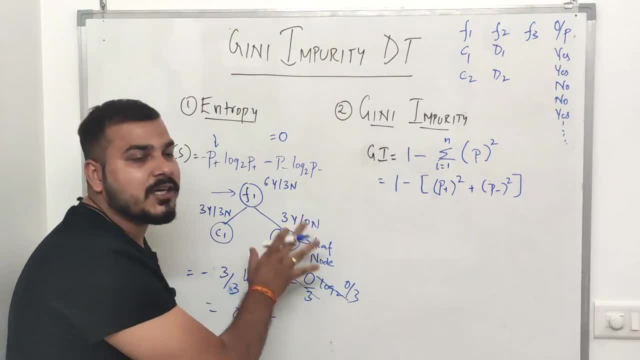 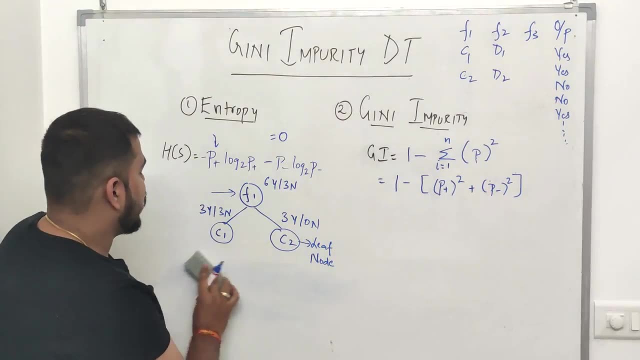 basically indicates that this is a pure split. Okay, Here we are actually getting a leaf node. Okay, So I'm just going to rub this quickly Now. the next thing is that what I'm going to discuss over here is suppose I consider, for this particular example, what should I do? Okay, 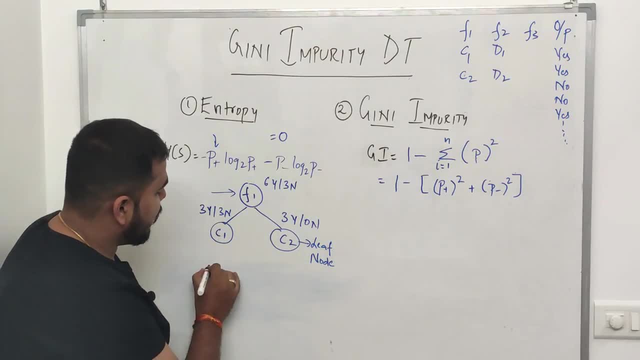 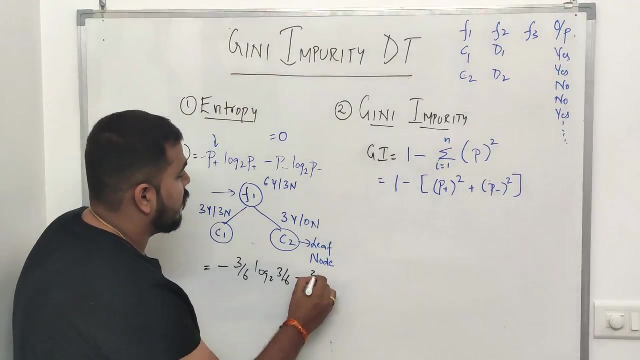 If I want to compute the entropy for this. So for this, what will happen? Again, minus P plus P plus is nothing but 3 by 6. Because I have 3 yes, 3 no's, 3 yes divided by total number of values, Then log of base 2 of 3 by 6, minus Okay, So. 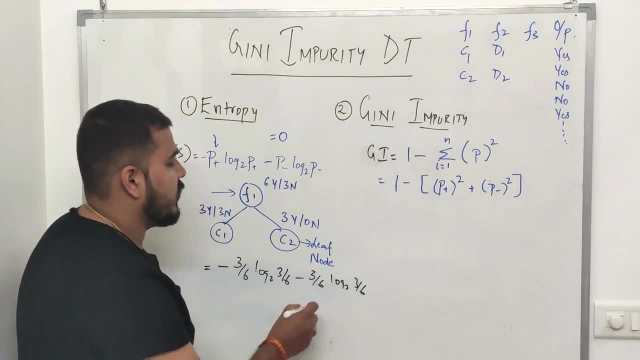 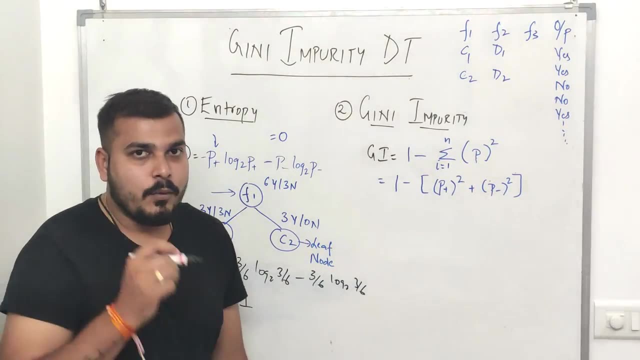 again 3 by 6, log 2, 3 by 6.. Because P minus is again 3, no's Right. So when I compute this, the value is actually 1.. Okay, Now why I'm saying the value is actually 1, understand in this? 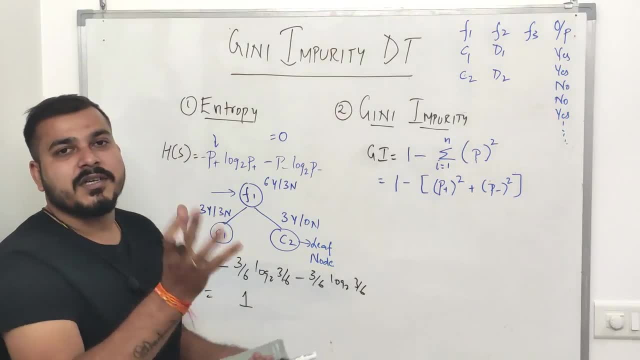 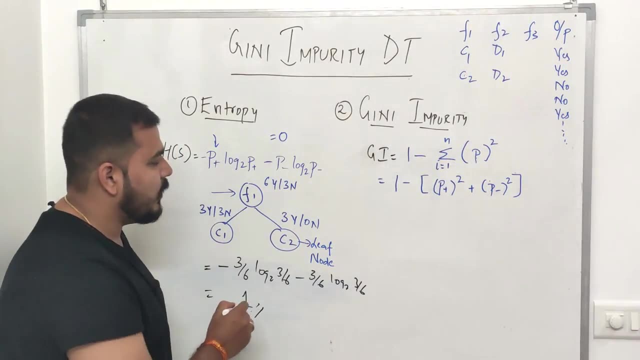 particular guys. Here it is completely 50-50% of probability. I have 3 yes or 3 no's Right- And if you try to do the computation, the complete computation, you will actually get a value of 1.. 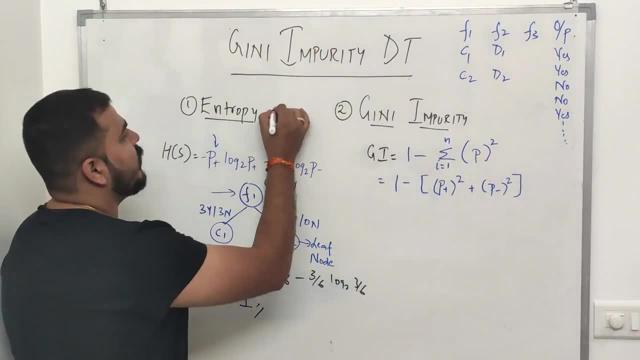 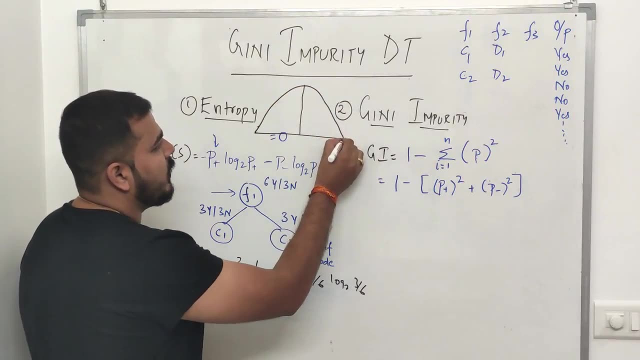 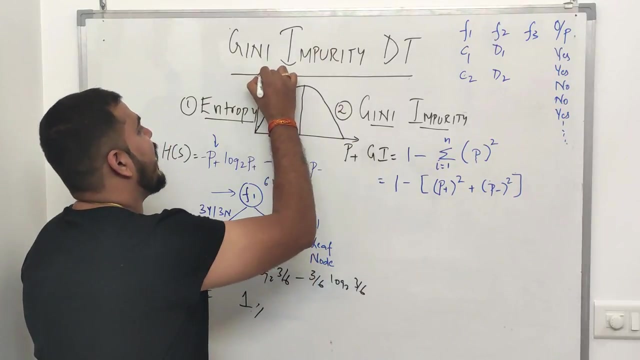 So by this it basically indicates that your entropy will be always ranging between 0 to 1.. Now what does this 0 to 1 basically mean? Suppose in my x-axis I'm going to take the value of probability of plus And here in my y-axis it's basically: 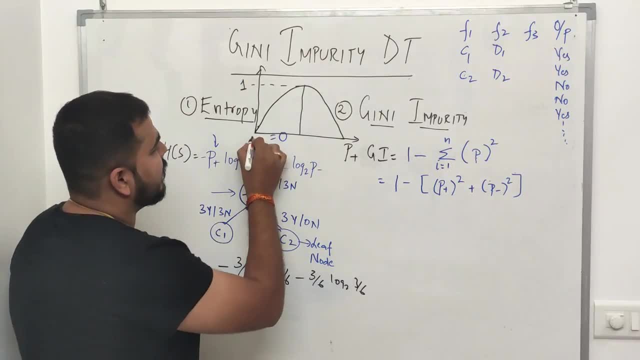 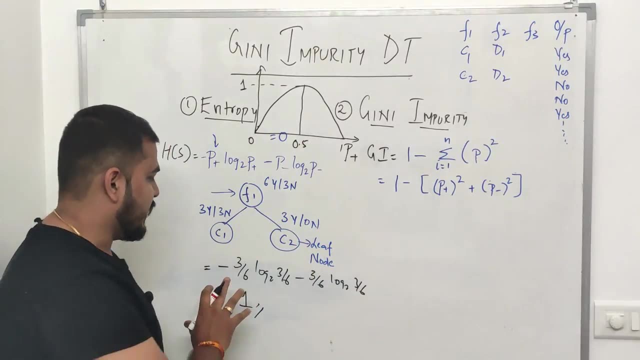 a graph. This will basically be 1.. Okay, And this is also between 0 to 1.. And this middle point is 0.5.. Okay, Now, what does this basically indicate? See this As the probability of plus value. 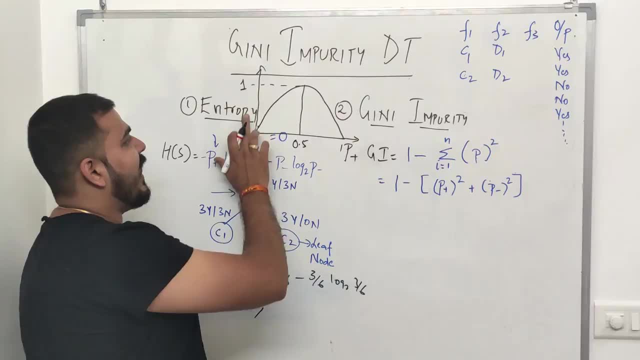 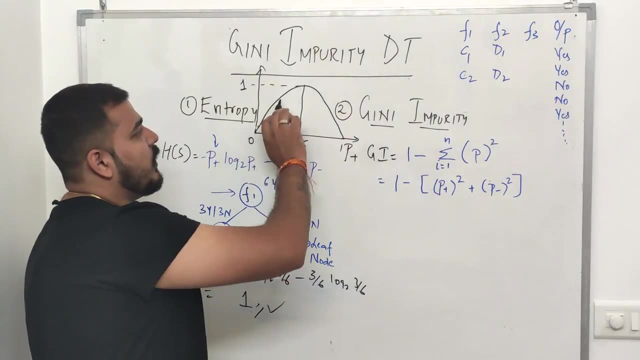 increases, Okay, Increases, So this value also increases. Now, what is this particular value? This value is nothing but entropy. Okay, So you can see that as this value increases, this will also increase At correct P. that basically means probability of plus value. 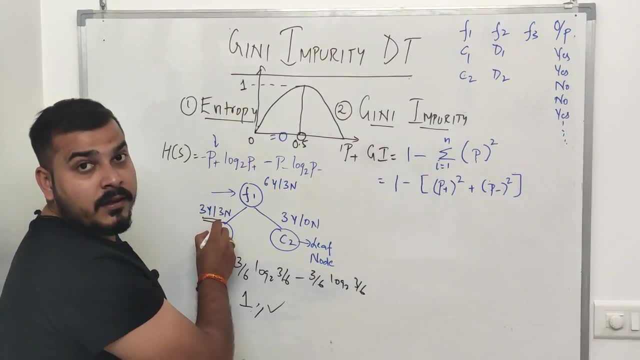 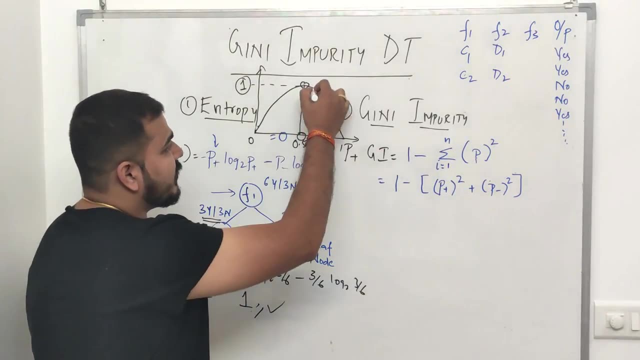 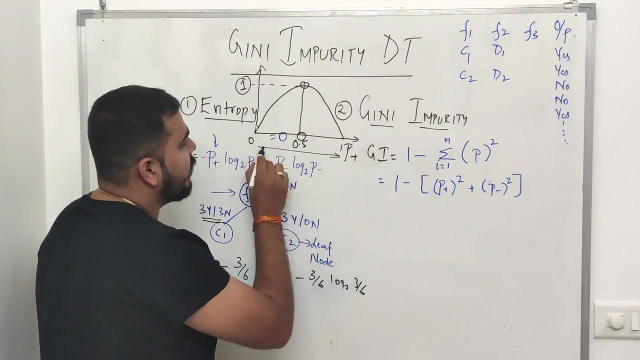 becomes 0.5.. In this particular case, it is 0.5.. Then your entropy will actually become 1.. Your entropy will actually become 1.. Then again, when it is reducing, when it is reducing, the value will actually decrease, Right? So between 0 to 1.. Right. 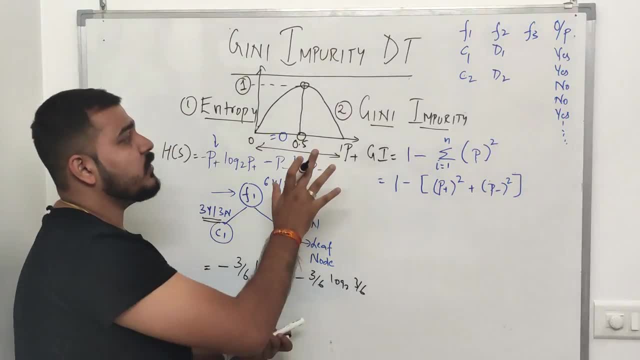 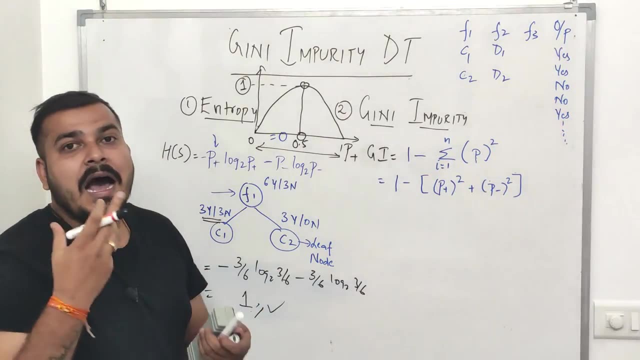 You can see that when the probability of plus is increasing, your entropy is also increasing. When your probability of plus is decreasing, your entropy is also decreasing. Okay, So that actually specifies how pure or impure a split is. Okay. Now, in this particular case, when I took this particular example, 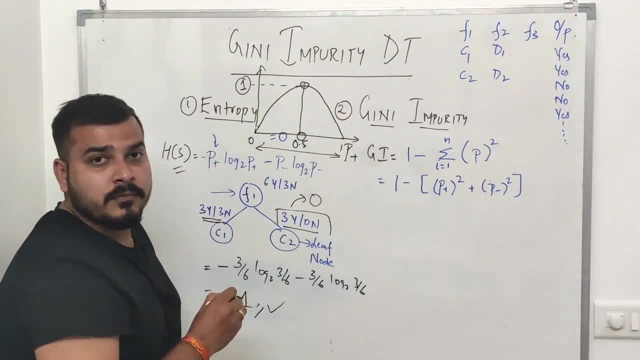 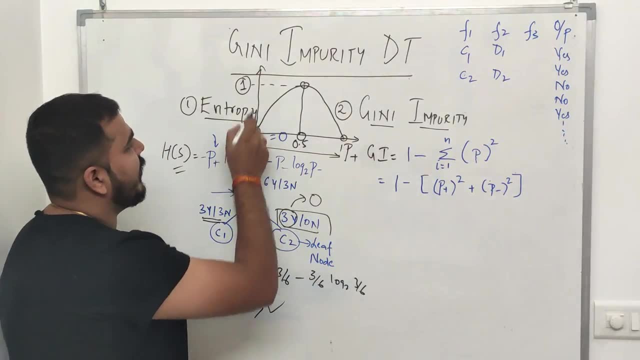 my H of S. it was actually 0.. Right, In this particular case I got 3 S, All was S. So, at this particular scenario, what is my value of H of S? It will be 0.. Now here I can basically say: 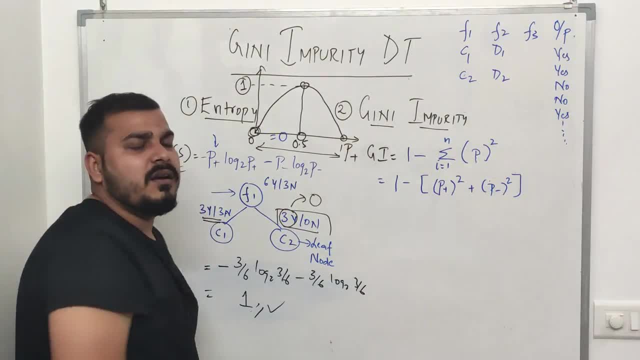 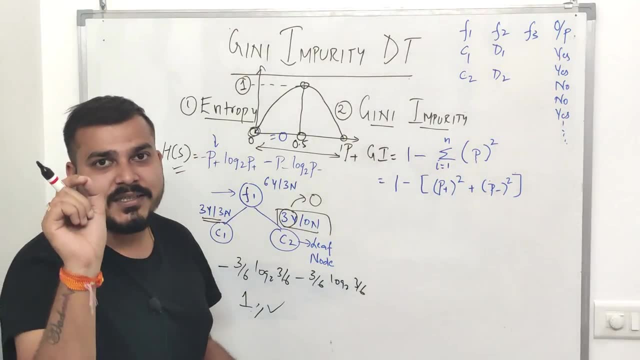 that this is a pure split. Now I have this wonderful explanation about entropy over here. It is working perfectly. Now why do we require Gini impurity? First of all, understand the formula, The formula difference between Gini impurity and this. let me just 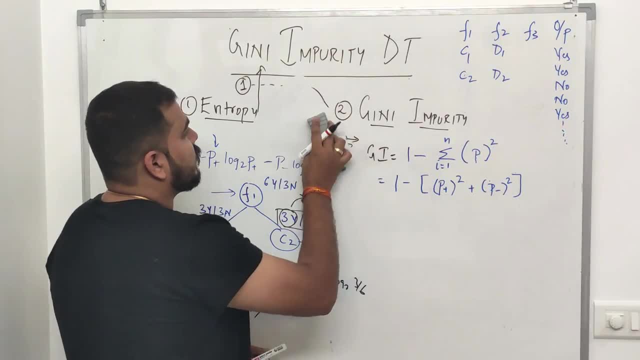 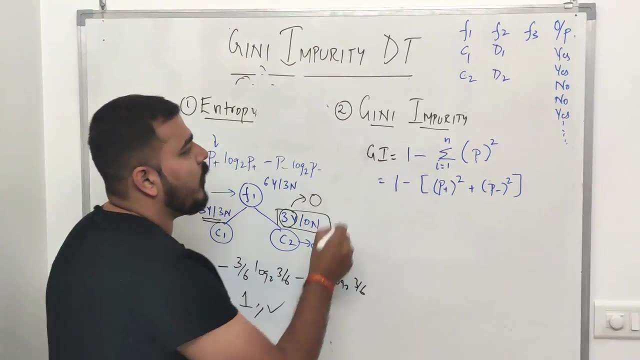 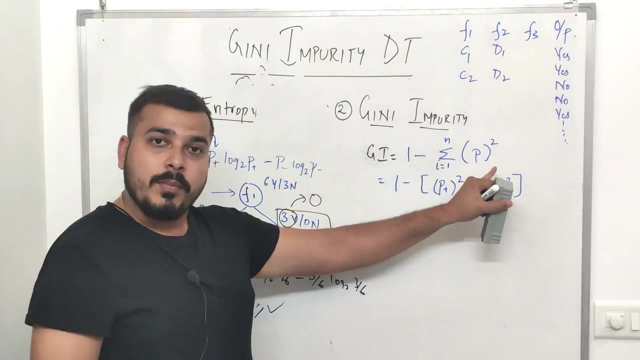 quickly rub it so that you will be able to understand it. Okay, Now the Gini impurity basically says that my formula basically becomes: 1 minus, summation of I is equal to 1 to N P square. Now this P square is nothing but probability of plus plus probability of minus. 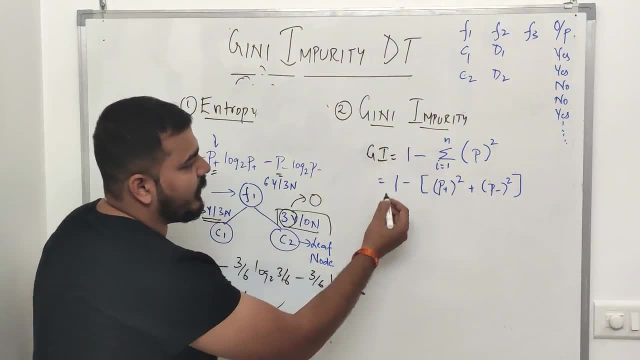 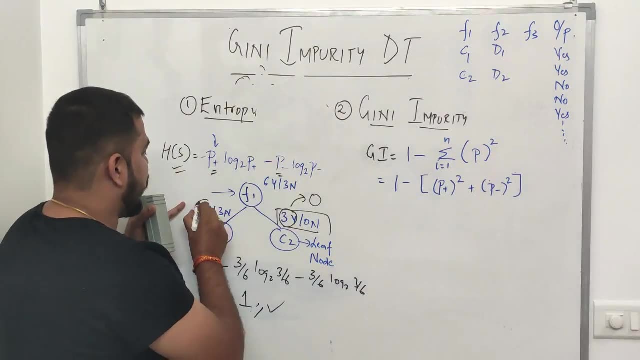 also. So both P plus and P minus. So this basically becomes: 1 minus summation of I is equal to 1 to N. So this is the formula. Now this P square is nothing but of P plus whole square plus P minus whole square. right now, suppose for this particular scenario, if 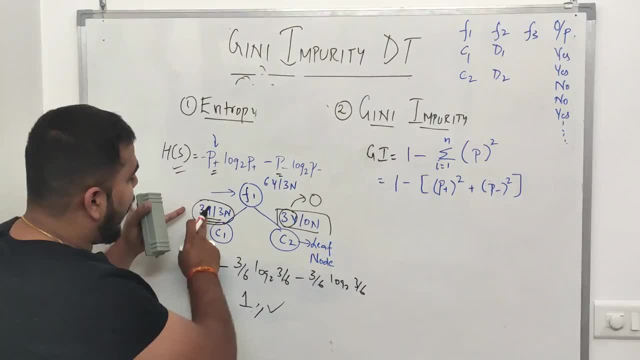 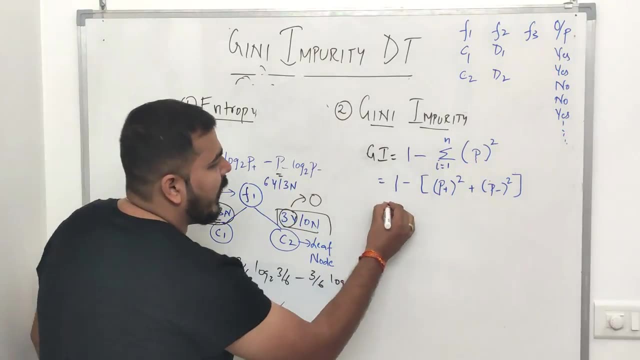 I want to compute for this particular scenario. if I want to compute, I saw that my entropy were having one value when I was in using this entropy formula. but if I use Gini impurity, what will happen is that this will actually become 1 minus. I know this is 50 percentage of probability, right? 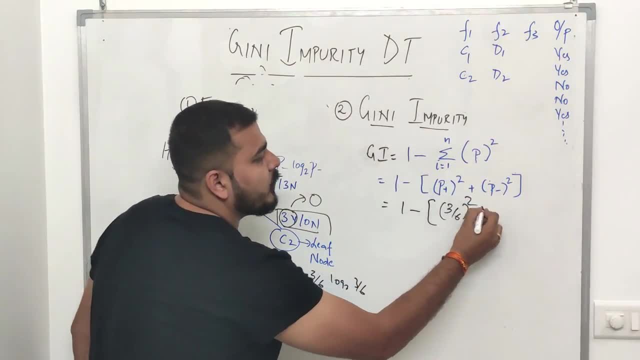 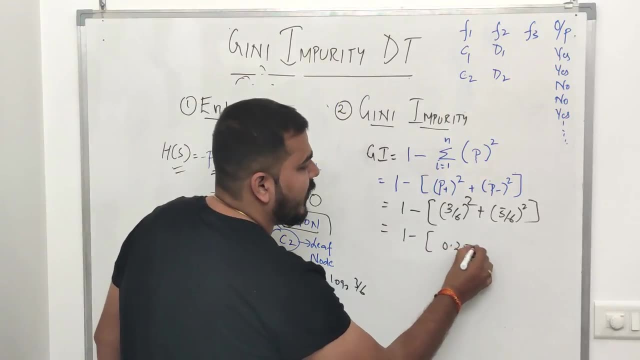 so P plus is nothing but 3 by 6 whole square plus P minus is nothing but 3 by 6 whole square. right now, if I try to compute this, this is nothing but 0.25 plus 0.25, which is equal to 0.5. now you, 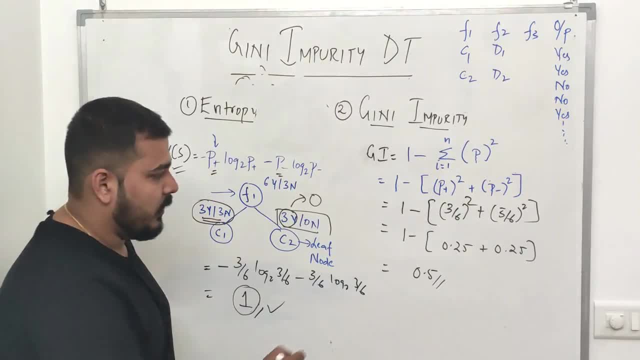 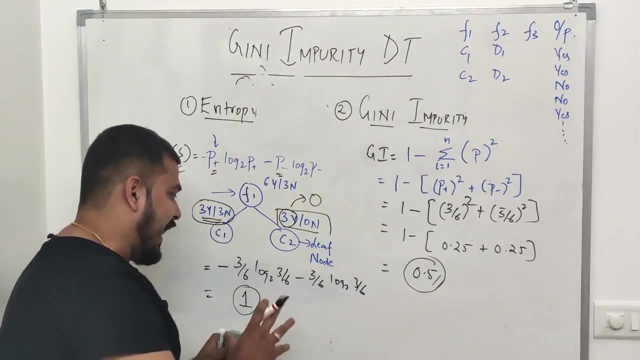 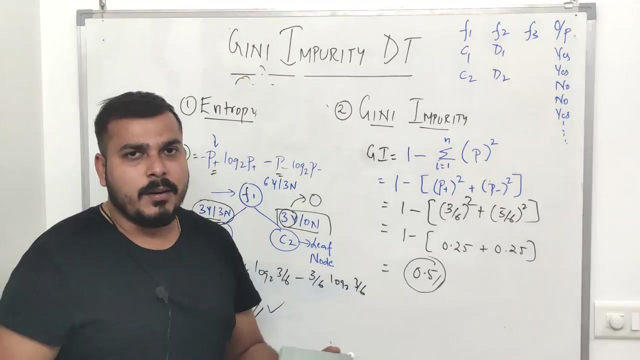 can see the difference. when I was using entropy, I'm getting as 1. when I am using this particular, the Gini impurity, I'm actually getting it as 0.5, right I? I see that my value is actually less when compared to the entropy. so you may be thinking: okay, Chris, it is fine, you are using this formula. 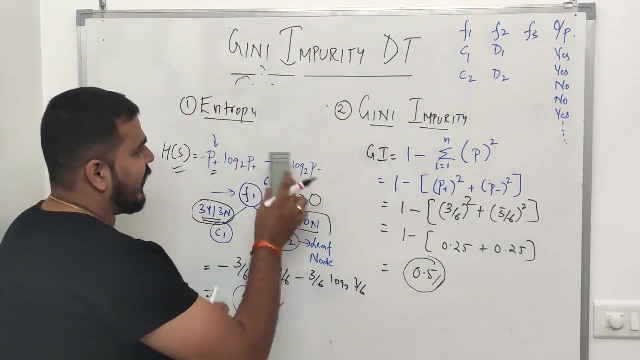 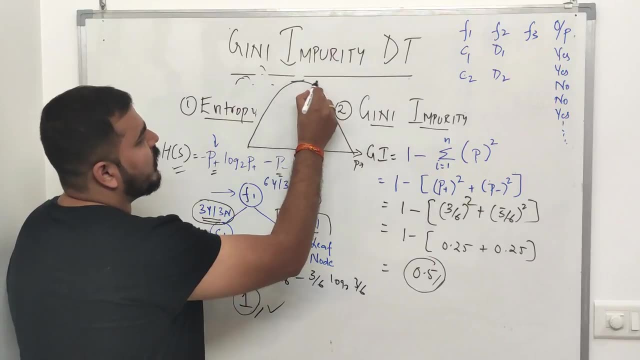 but what is the main use? right and understand, guys, if I again you are using this formula. but what is the main use? right and understand, guys, if I again, we recreate that particular diagram which I actually created, like this: with respect to probability of plus, this value is with respect to entropy. right, the same diagram, if I construct. 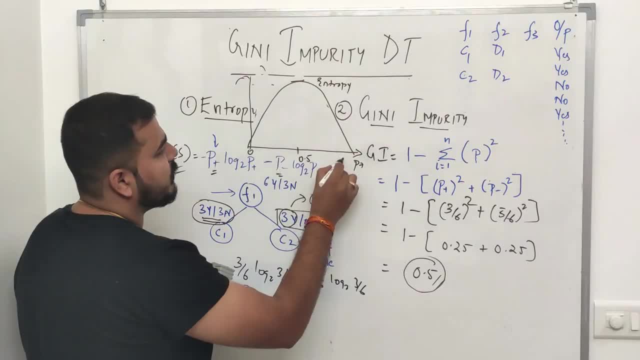 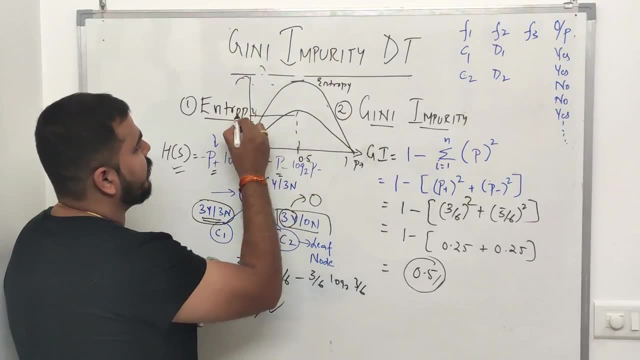 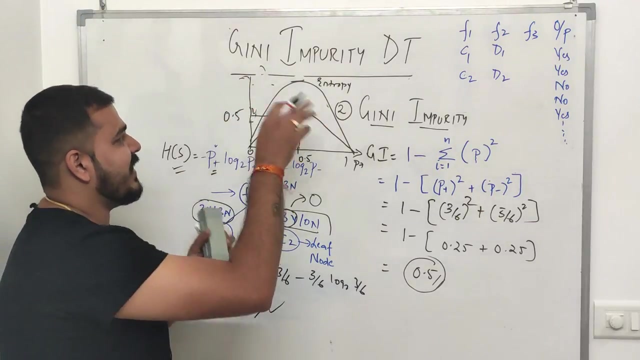 for Gini impurity, and this is 0.5. right, this will be ranging between 0 to 1. this value will actually become like this. the diagram will actually become like this, and this will be 0.5. okay, I'm just going to rub this quickly. sorry for the diagram. 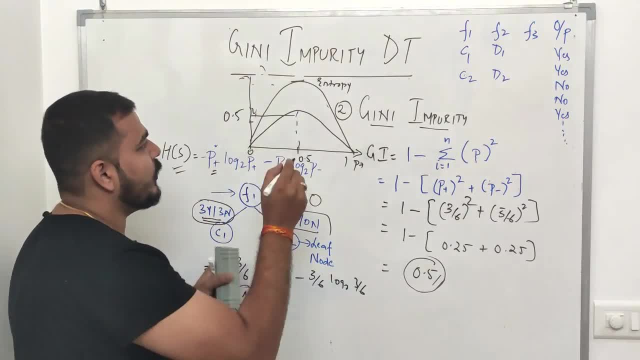 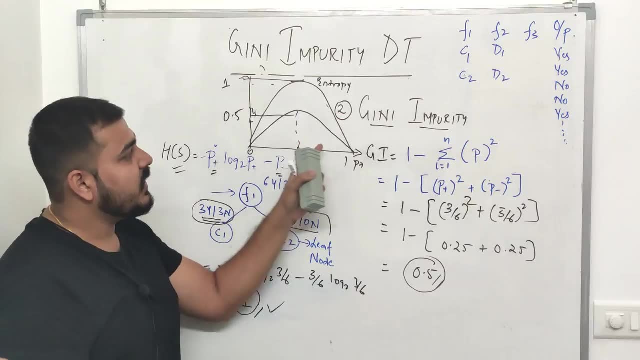 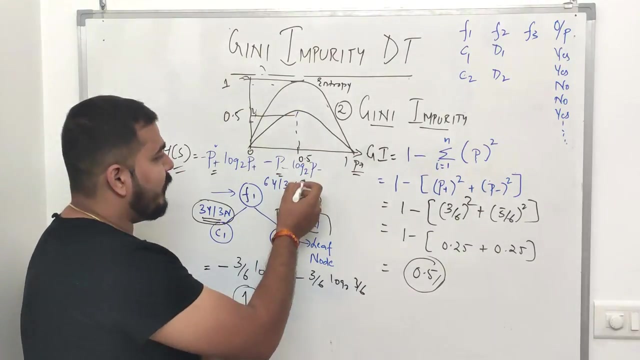 I'm messing it up over here itself, but just understand, we need to understand this and this is actually one. okay, now, this particular smaller diagram that you see is basically for Gini impurity. this basically says that when your probability of plus or probability of negative, is increasing and when it becomes 50%, like 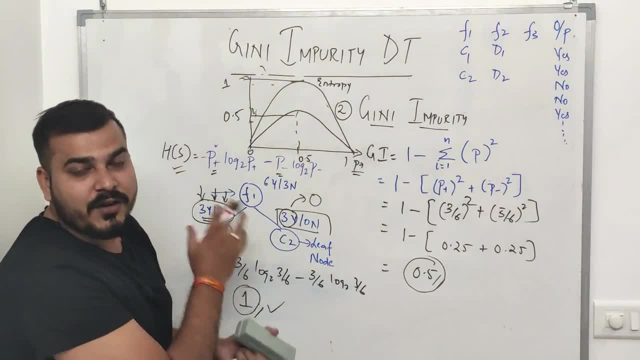 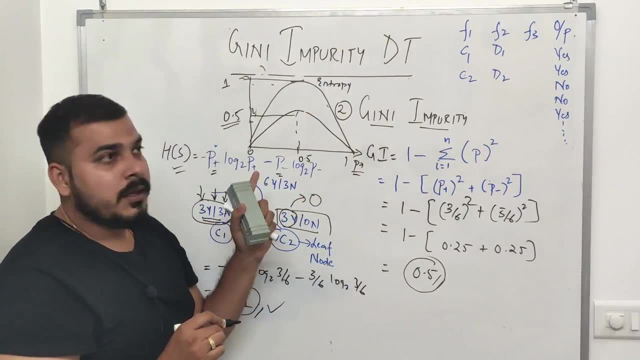 this, like this scenario: when you have 3s or 3 nos or 5s or 5 nos, in this particular scenario, your maximum value will go till 0.5. then it will actually reduce, but in the case of entropy, the maximum value was actually going till 1. the entropy value was. 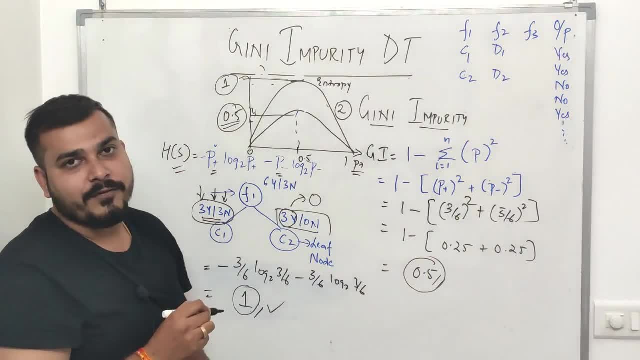 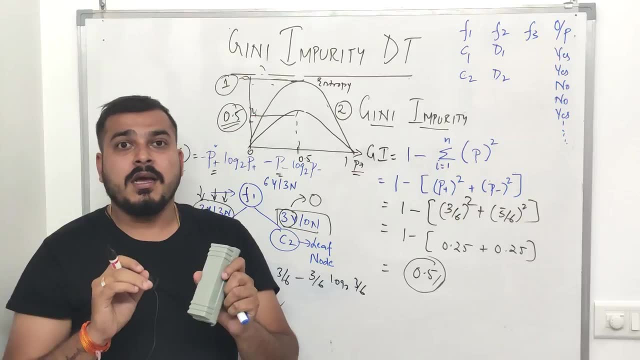 going till 1, whereas in Gini impurity the maximum value is going to 0.5. okay, now the major thing: why do we use Gini impurity in many of the state-of-art algorithms? Gini impurity is basically used in some of the ensemble techniques where random forest XGBoost are kind of used over. 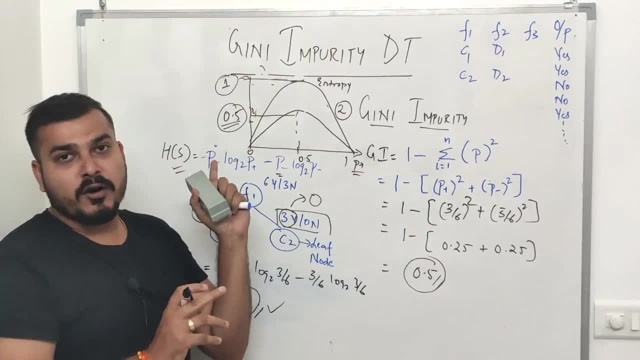 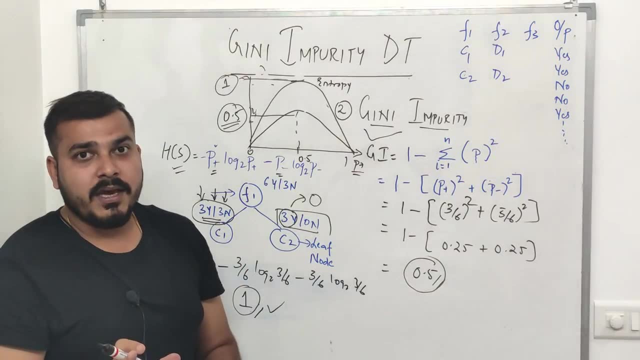 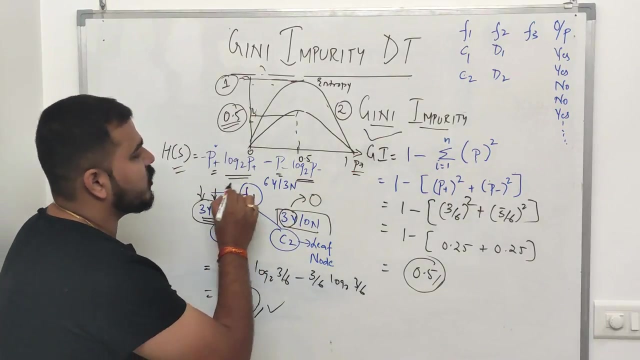 there. they are taking as Gini impurity as the parameter instead of entropy. the reason is that this is computerized, computationally efficient. okay, this takes a shorter period of time for execution. why see this formula, guys? log base 2, log base 2 usually if you want to do the logarithmic calculation. it. 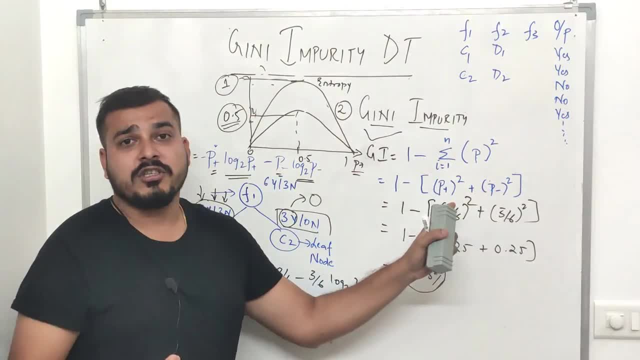 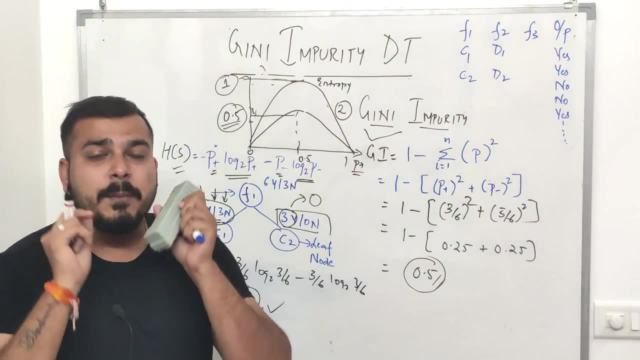 usually takes some amount of time, but in this particular case we don't have those kind of computations right and you can see basically this particular graph. this is a very, very good interview. question, guys, they may probably ask you: why do you use Gini impurity? why do you use entropy? in which scenario? because after this: 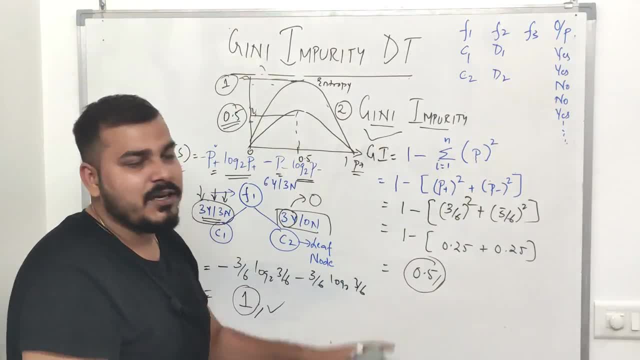 all you have to do is use the information gain formula right to compute all the values right. so this is the basic difference between entropy and Gini impurity. okay, and this is how you have to explain the interview. also, you have to make sure that you explain them this particular diagram, the 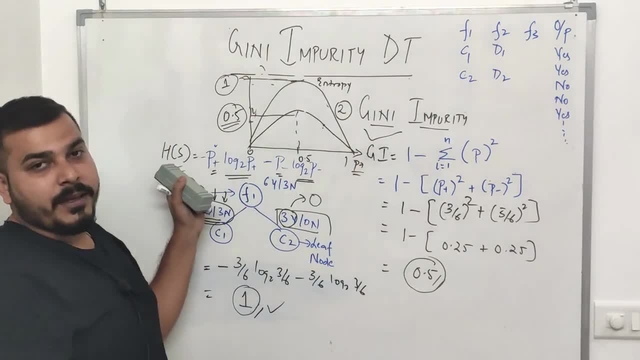 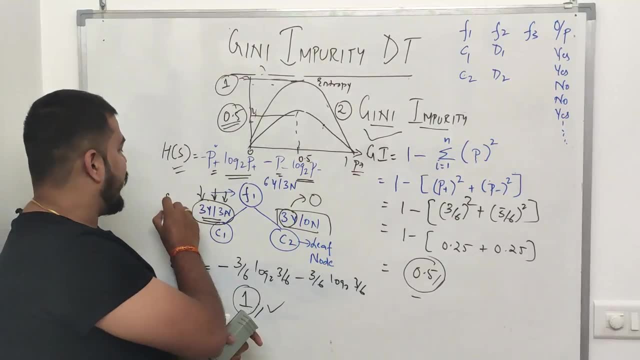 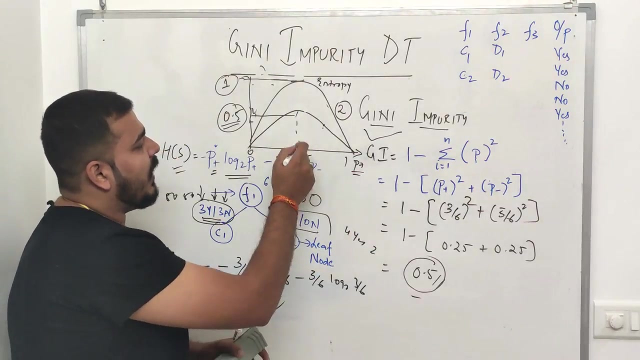 inner diagram is for Gini impurity, the outer diagram is for entropy. and you should also say that when your probability of plus value is increasing. increasing basically means: suppose here I have fifty, fifty percent scenario, suppose I have four yes, two no's for that particular value. it will be increasing 4s after reaching some specific point. 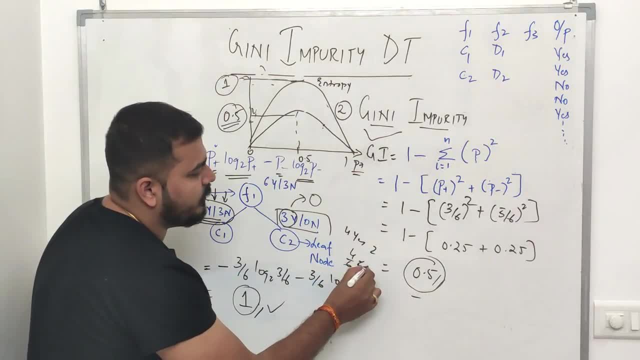 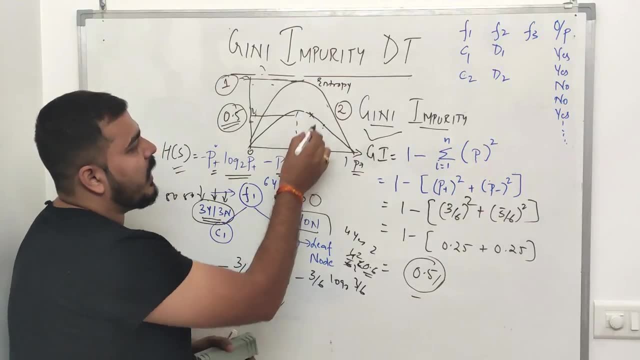 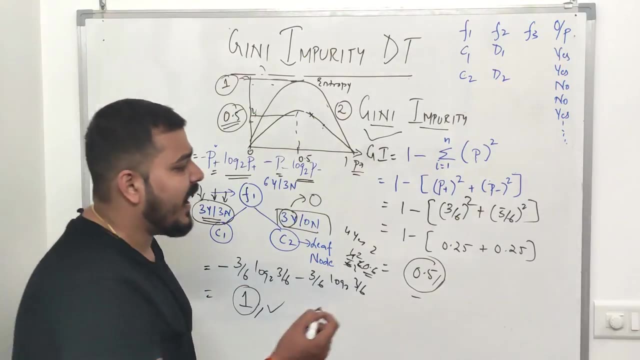 in this. if i calculate 4 by 6, this is less than you can say 2 by 3. this is actually 0.6. 0.6 basically means in this particular point, at this scenario, the linear impurity will be decreasing. if it is within this particular block, it will be increasing till 0.5. the maximum increase will be: 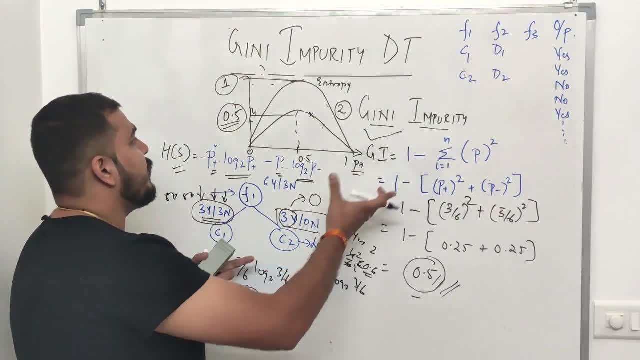 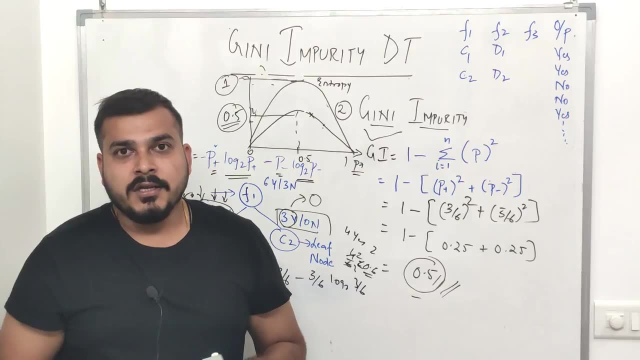 only till 0.5. after that you use linear impurity or entropy. but and after that what happens? information gain is actually calculated and the split actually happens. so yes, this was all about this, particular videos, guys. in my next video over here i took an example of category feature. 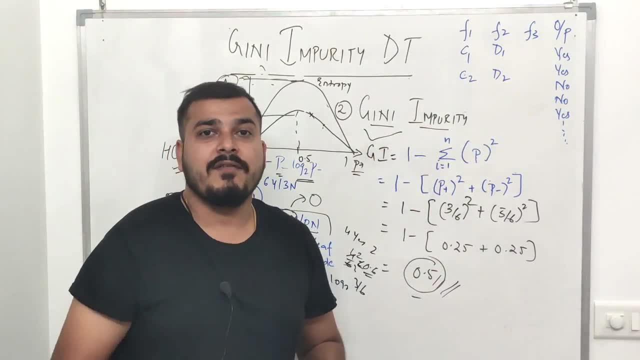 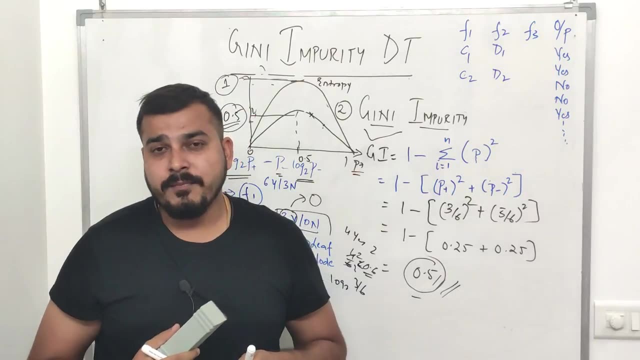 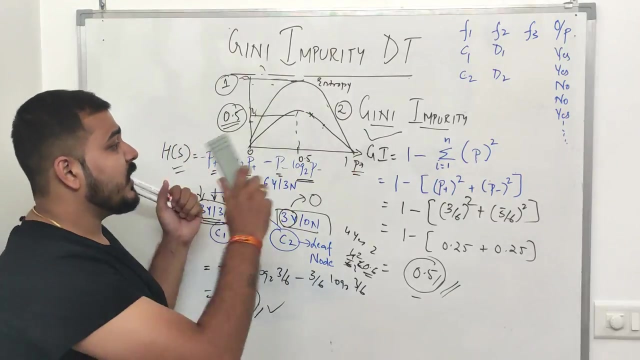 what if in my features i have only numerical values? how do decision tree actually split it? we need to have a look on to that also, so that will be coming in my next tutorial. so i hope you like this particular video, and many of you had actually asked that. how does guinea impurity actually work? so this was all about this particular 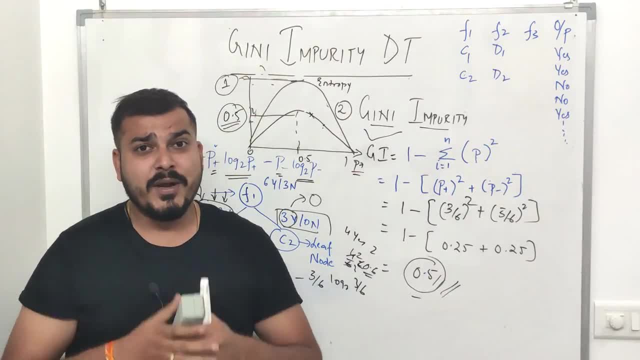 explanation. so i think i hope you like this particular video. if you have any queries, please do comment down in the description box- sorry, in the comment section itself. i'll be happy to answer all the questions that you have. so yes, this was all about this particular video. i hope you like it. please do subscribe the channel if you have not already subscribed. i'll see you all in the next video.